mm is cube size. So on the perfect day the soil sample will be sieved through uniform size ofercal sieve of 4.75 mm. Solijk analysis is done for coarse grain soils which are 글랍 4.75 mm sieve. This arose over a period of some 2 .2 years and will be sung over other. 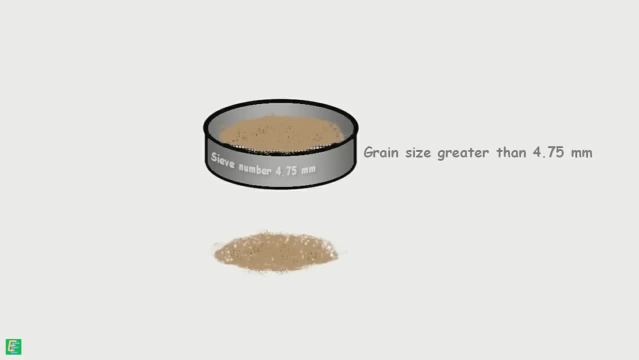 is retained on the sieve. This portion is called gravel fraction. The portion of soil which contains particle size less than 4.75 mm pass through the sieve. This portion is called sand fraction. This way, coarse-grained soils are divided into two categories. One is gravels having grain size greater than 4.75 mm, and second. 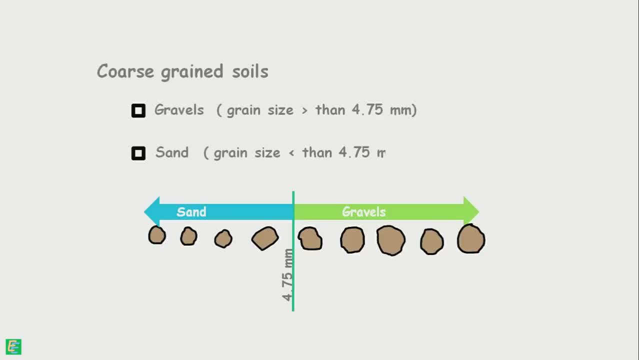 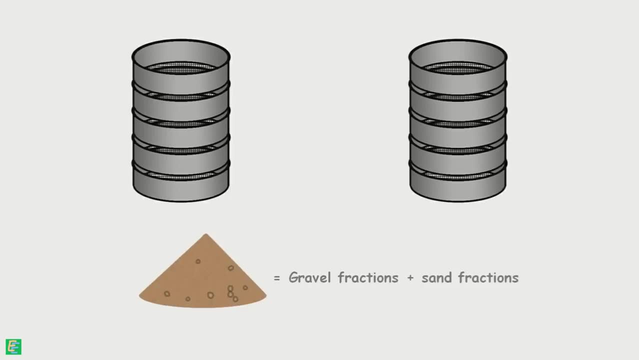 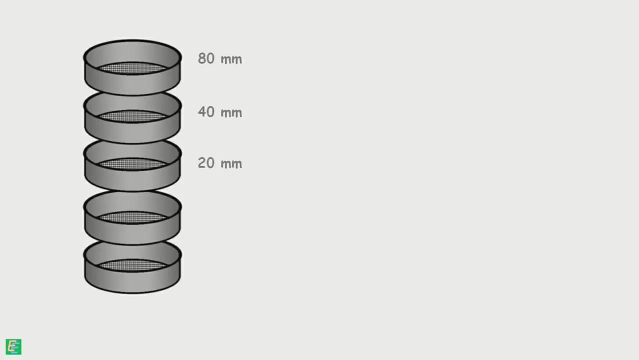 one is sand having grain size smaller than 4.75 mm. So for sieve analysis of our sample we need two set of sieves, One for gravel fractions and another for sand fractions. For gravel fractions we require sieves of sizes 80 mm, 40 mm, 20 mm, 10 mm and 4.75. 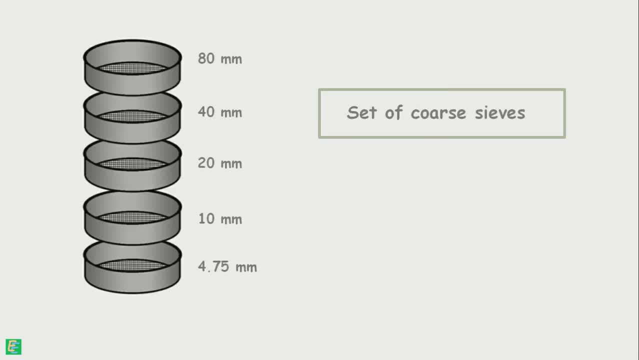 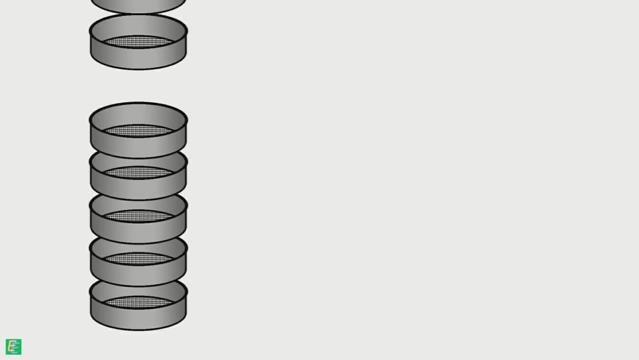 mm. This set is called set of coarse sieves as it sieves coarser part of coarse soils. Second set of sieves for sand fractions consists of sieves of sizes 2 mm, 1 mm, 600 micron, 425 micron, 212 micron, 150 micron and 75 micron. 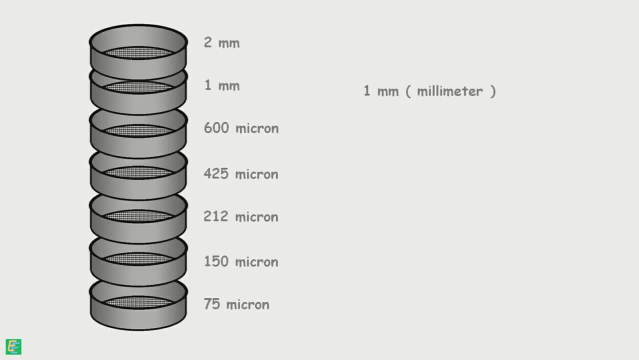 If we didn't mention, then 1 mm, that is mm, is equal to 1000 micrometer, which we denote as micron. So 1 mm is equal to 1000 micron. So here 600 micron is actually 0.6 mm. 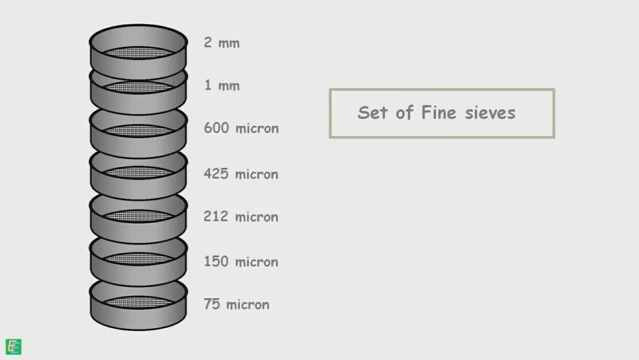 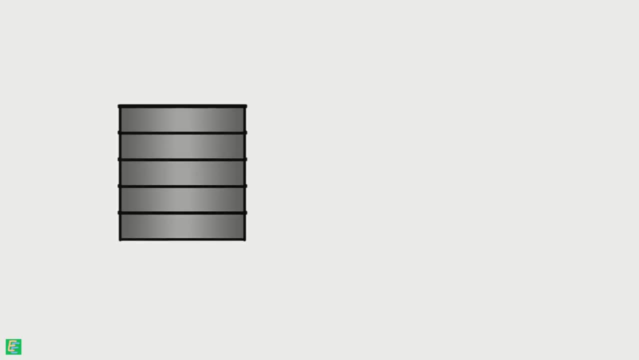 This set of sieves is called set of fine sieves as it sieves finer part of coarse soils. The sieves are stacked one over the other With increasing size of sieves. The sieves are stacked in the size of their mesh openings, from bottom to top. 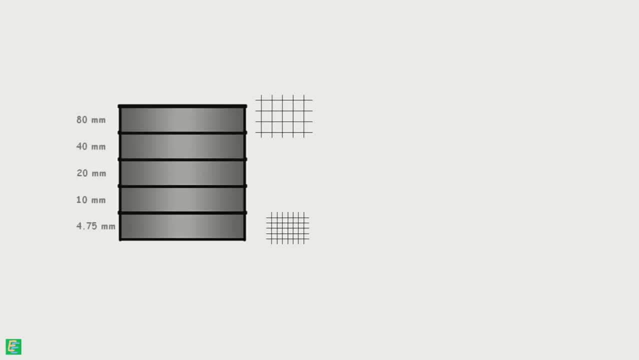 Which means the sieve of the largest opening is kept at the top. The pan which has no opening is placed below the bottom most sieve. The soil sample is placed in the top sieve and the lead to cover this arrangement is placed over the top most sieve. 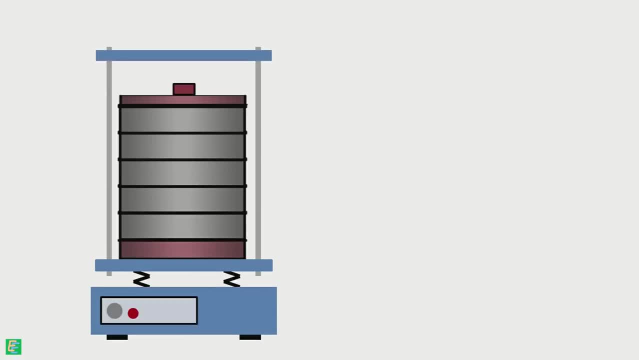 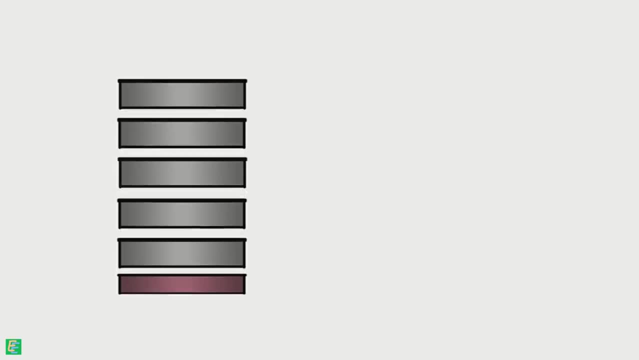 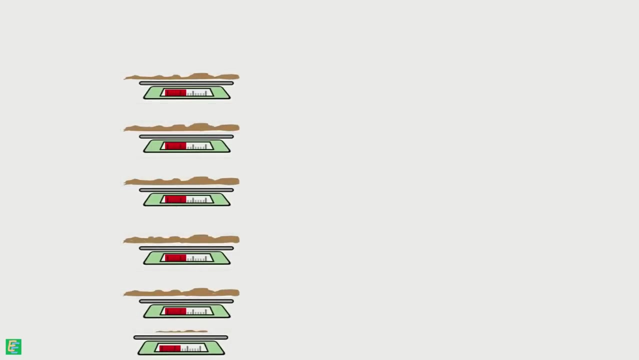 The whole arrangement is then placed on a mechanical shaker and shaked for 10 minutes. Then arrangement is taken out and the amount of soil retained on each sieve and pan is weighed with the accuracy of 0.1 gram. Let's say the weights retained on the sieves are W1, W2, W3, W4, W5 and W Pan. 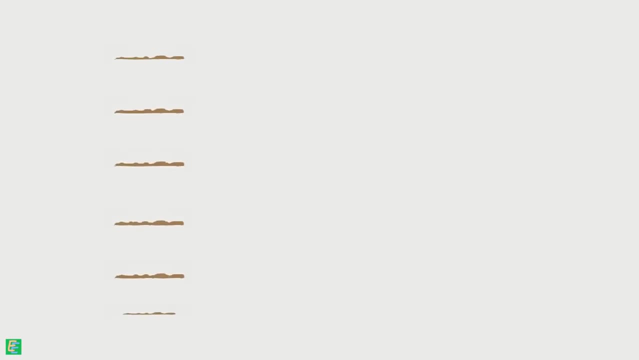 Then we calculate the percentage of amount of soil retained on each sieve as weight of retained soil on the sieve. Thereas, to calculate the total amount of soil retained on each sieve is: W1,W2,W3,W4,W5,WPan. 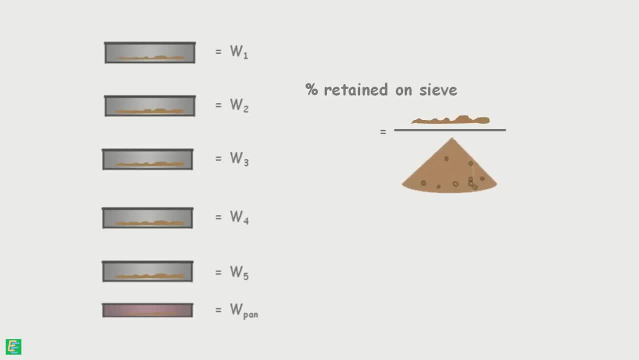 Then we calculate the percentage amount of soil retained on each sieve as weight of retained soil on the sieve divided by total weight of soil, soil sample multiplied by 100. This way we know what percentage of total weight is retained on a particular sieve. Percentage weight retained on the first sieve is W1 divided by capital W. 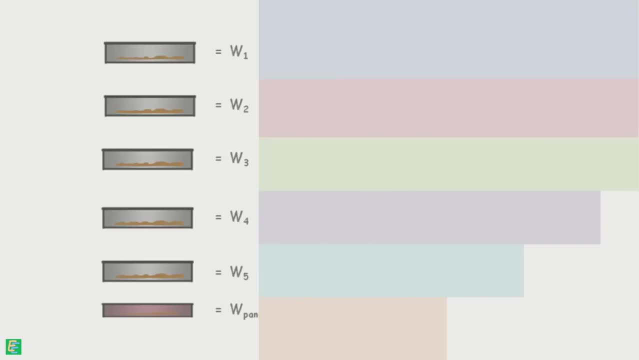 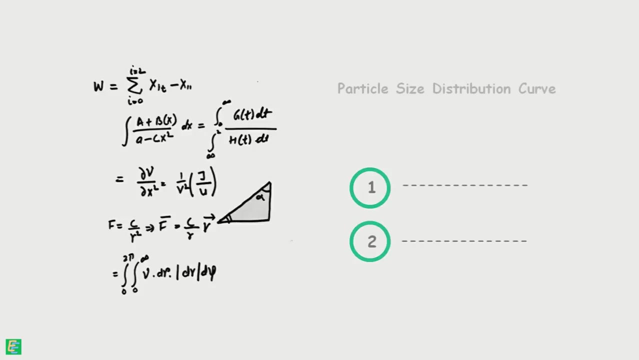 multiplied by 100.. Let's say these percentages as P1, P2, P3, P4, P5 and Ppan. For calculation purposes and to determine some important characteristics, we also calculate two values. First one is cumulative percentage retained. Let's write our calculations in a table. 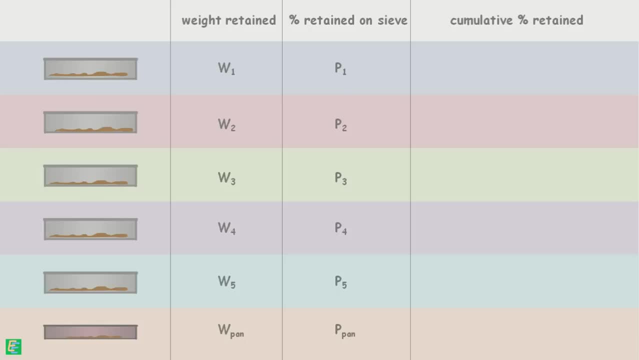 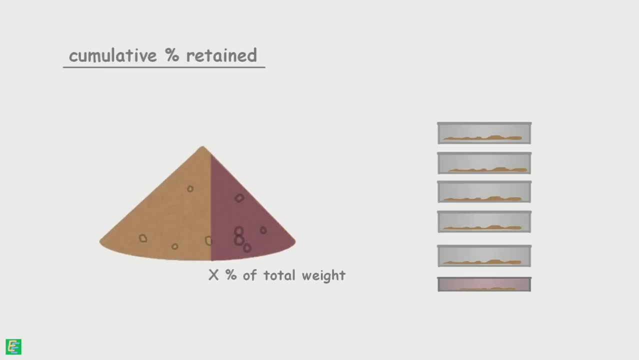 Now, cumulative percentage retained of any sieve is the percentage weight retained on that sieve plus all percentage weight retained of all the sieves above it. Cumulative percentage retained is the total percentage amount of soil which could not pass the particular sieve. In other words, this percent amount of soil has grain. 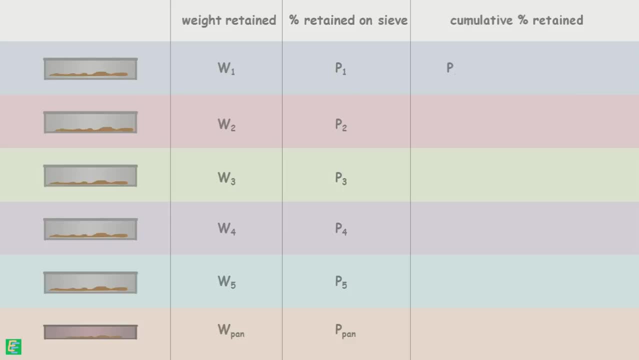 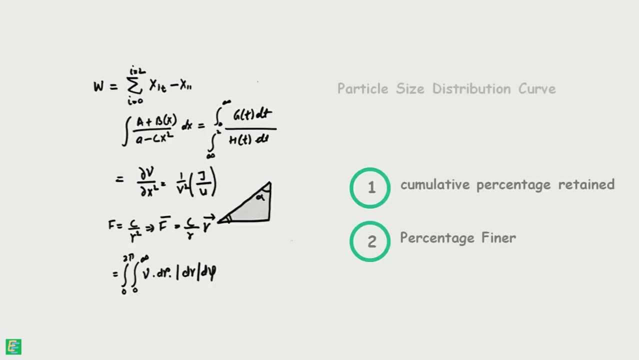 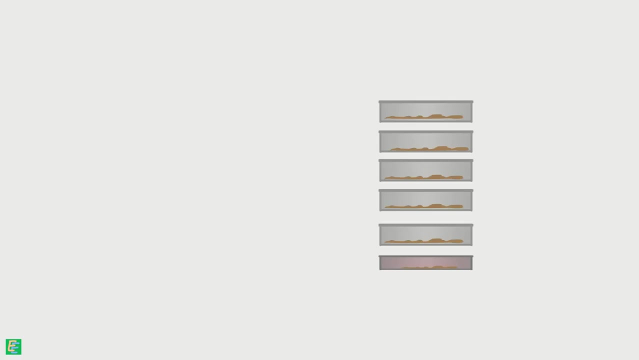 size greater than the sieve number. So let's calculate the cumulative percentage retained for each sieve. Second value we calculate is percentage finer, using which we plot a graph called particle size distribution curve. Percentage finer, as name suggests, is the percentage amount of soil which is finer than the grain size of the sieve. So let's calculate cumulative percentage. 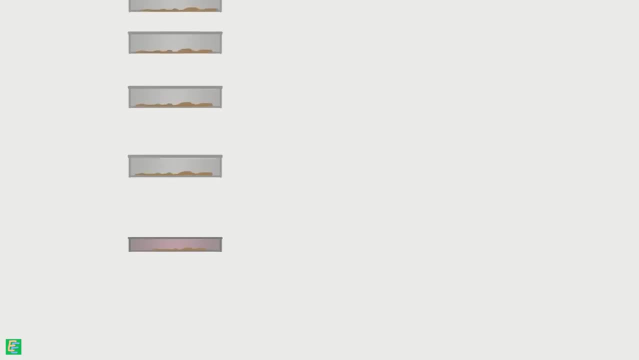 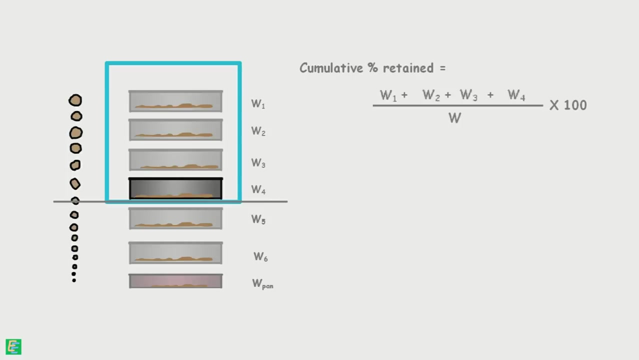 than a particular sieve. Consider any sieve from the stack. The amount of soil above this sieve is coarser and its total weight in percentage of total soil. sample weight is cumulative percentage retained on this sieve And the amount of soil below this sieve is finer portion of the sample which has particle size.